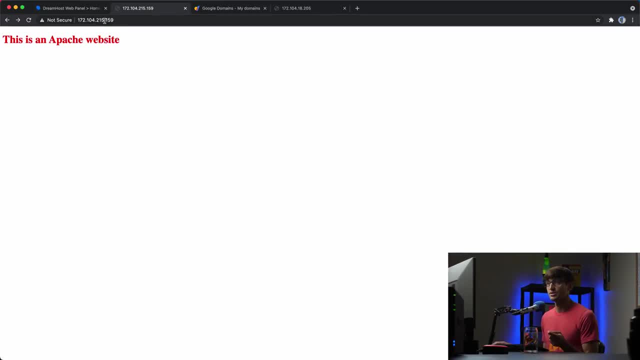 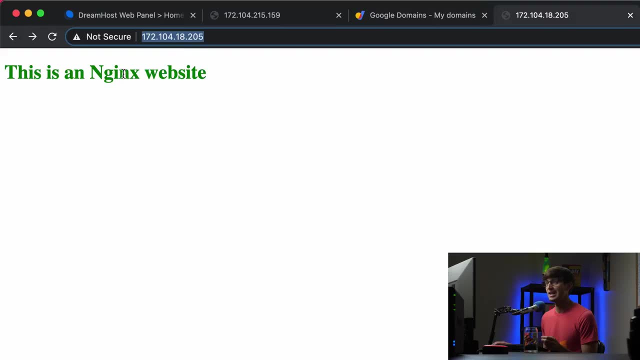 Okay, so I have two websites at IP addresses: This Apache website at this IP address ending in 159, and over here in this other tab, an NGINX website ending in this IP address, 205.. Okay, and the goal- The goal by the end of this video is to back over here. I have a domain name with dream host. 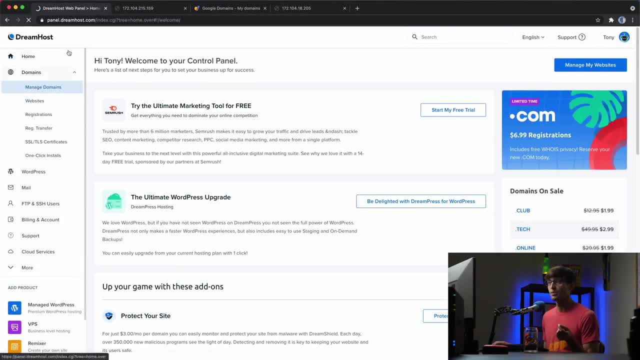 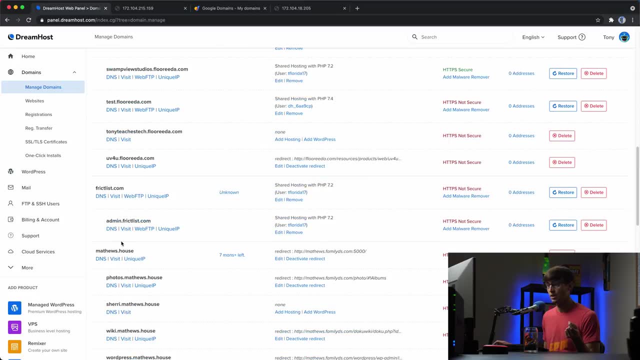 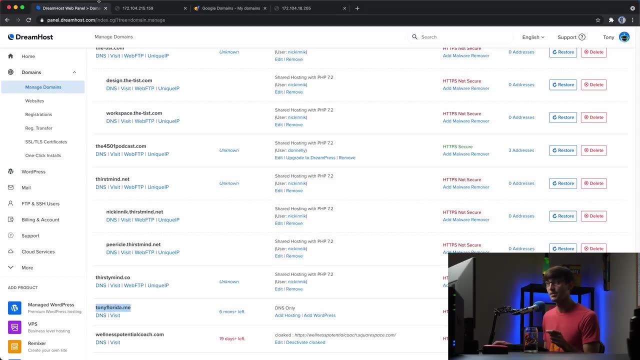 Okay, let me show you that in my domains- here I want to point one of my dream host domain names, specifically Tony. Where is it? I'm scrolling too fast, Bear with me. I want to point TonyFloridame to this IP address. 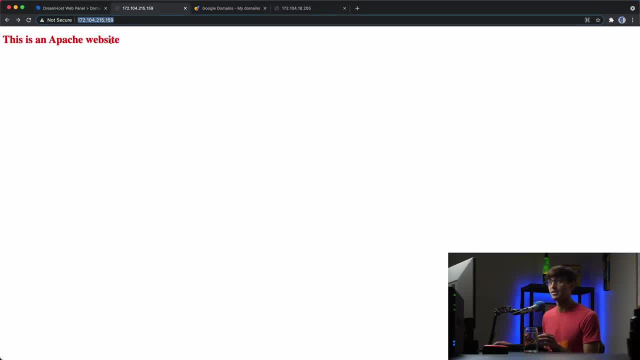 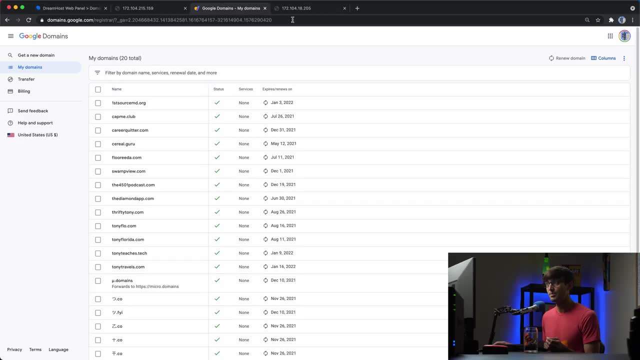 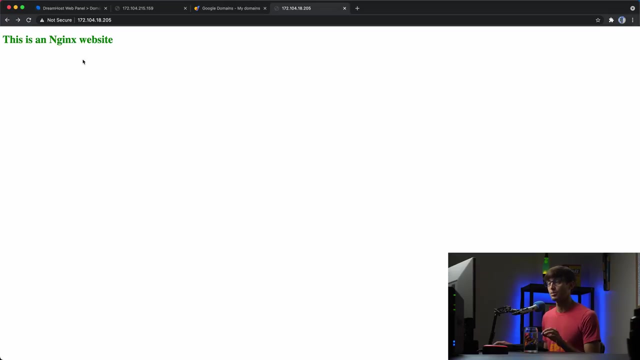 So instead of going to the IP address, you go to TonyFloridame, and then we see this show up. And over here, with Google Domains, I want to have CareerQuittercom point to this IP address. So instead of, you know, typing the IP address, we go to CareerQuittercom and this same website shows up. 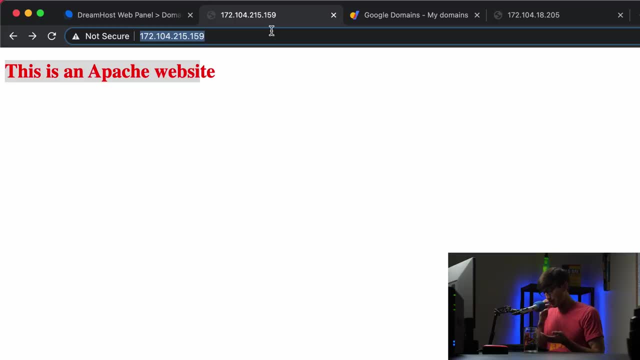 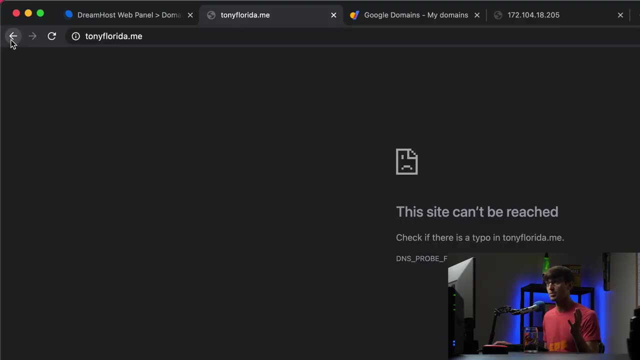 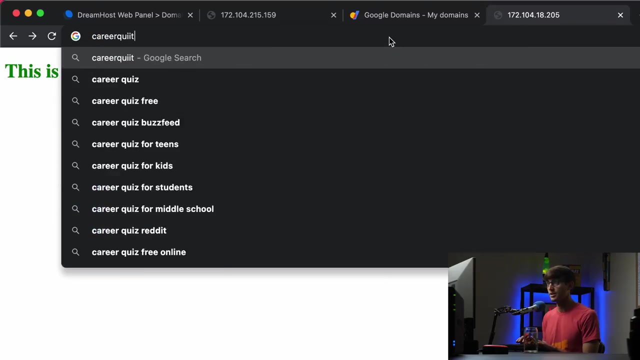 So let me show you right now: if we go to TonyFloridame, there is no website hosted here. There's nothing at this point right. And the same thing for CareerCAOme, CareerQuittercom- spell that wrong. Q-U-I-T-T-E-Rcom. 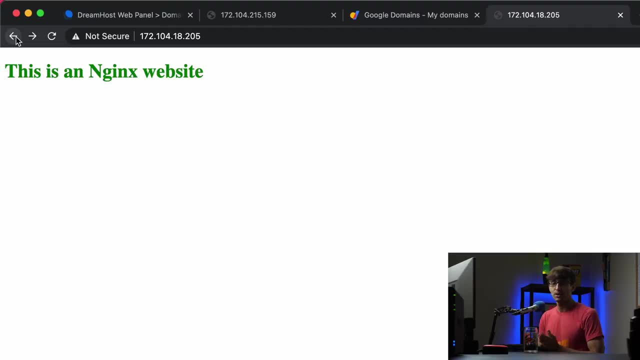 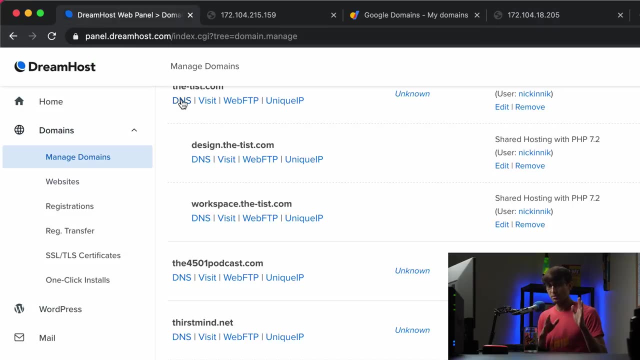 There's also no website hosted here, So let me show you how to set up your DNS records so that we can point those domain names to those IP addresses In dream host. again, remember: this will work for GoDaddy, This will work for Namecheap- any of your hosting providers out there. 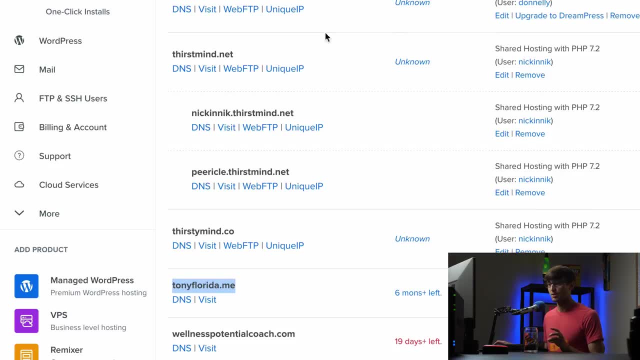 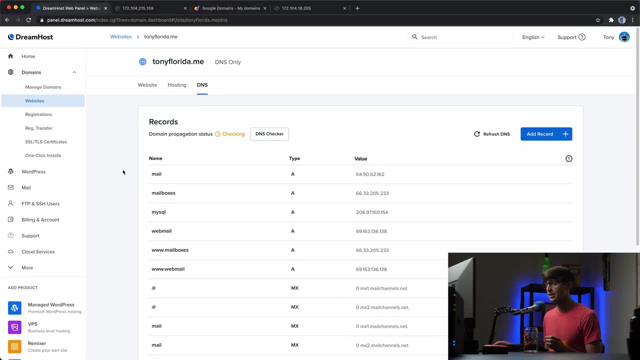 You just need to find the DNS section for your domain name. So for me, that's right here. Here's my domain name and here's the DNS. What I want to do in here is add in a DNS record. okay, The DNS record is going to be of type A. 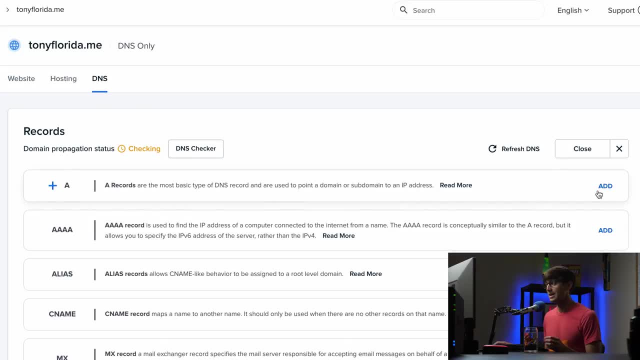 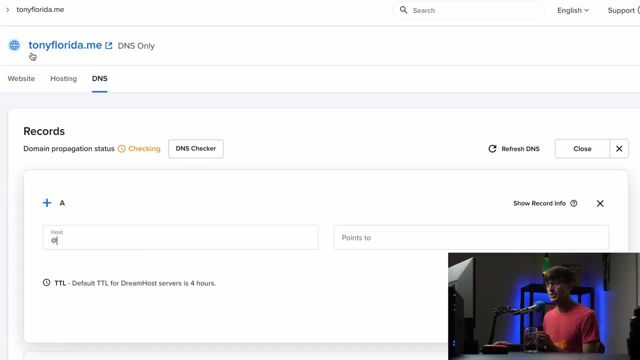 There's multiple different types of DNS records, but we want an A record, So let's add an A record. The host, the convention for this is the at symbol to as a shorthand for the actual domain name, and that's going to point to that IP address. 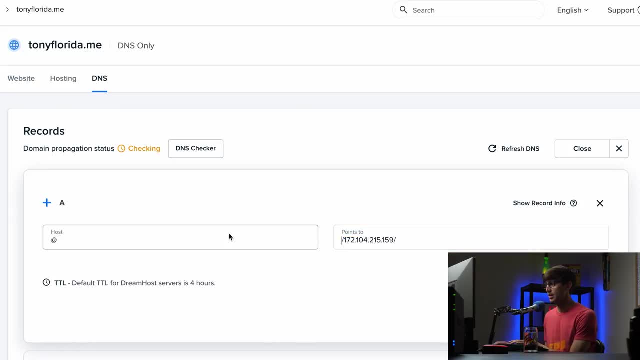 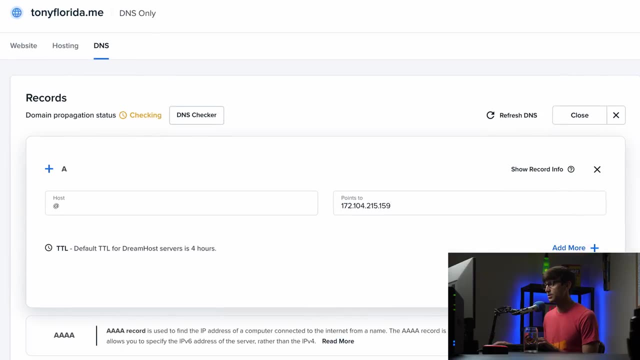 So let me copy this IP address, paste it here. We don't want, we just want the numbers, The numbers and the dots. So tonyfloridame is going to point to this IP address, So we will do one more record as well. 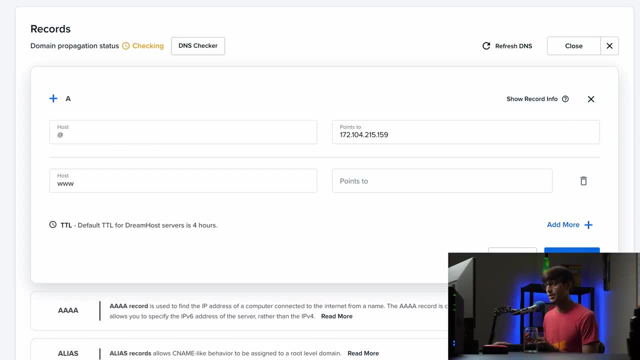 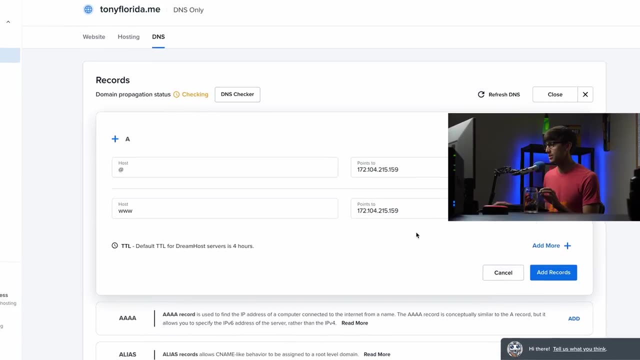 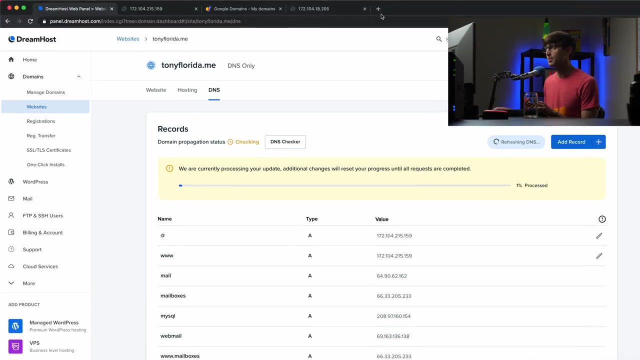 We want wwwtonyfloridame to point to that same IP address and we'll get rid of all that other junk, just so we have the IP address. Okay, so let's add those records and they're doing the updates. And while that's happening, let me show you something cool. 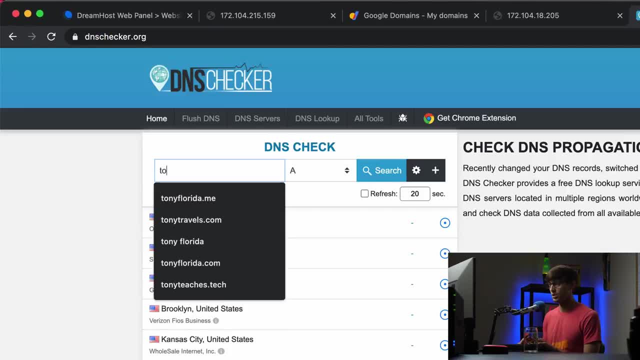 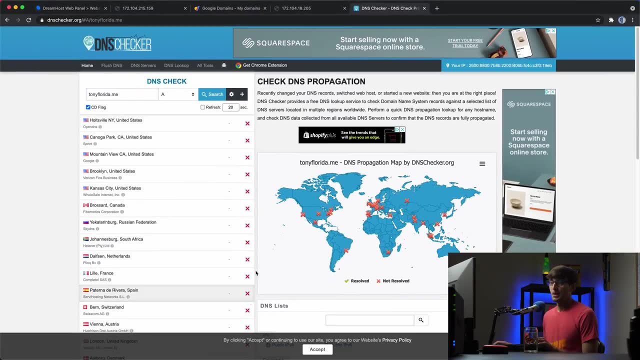 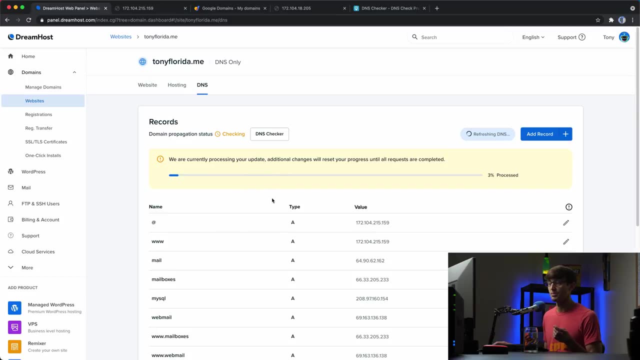 So if you go to dnscheckerorg, you're going to see this. So if you go to dnscheckerorg and we go to tonyfloridame, look at the A record for tonyfloridame. there are no. the DNS servers out there around the world don't know about that yet, because DreamHost is still processing our updates. 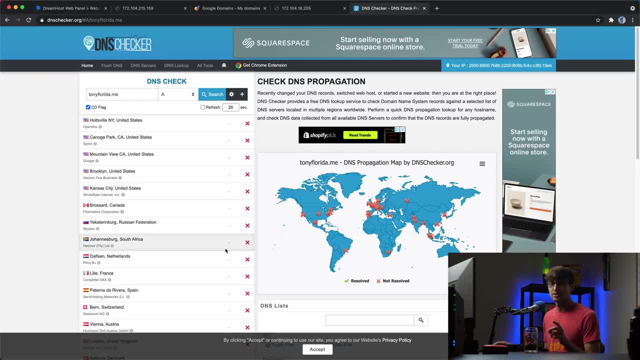 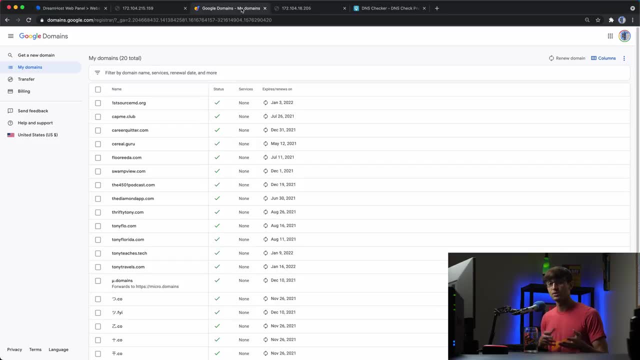 So we'll keep that in mind. We'll come back and look at this and see if the status changes, But in the meantime, while that's happening, let's do the same exact thing, but just to show you a different example, for Google domains. 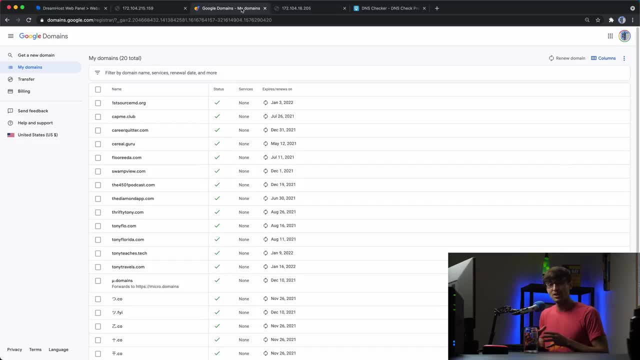 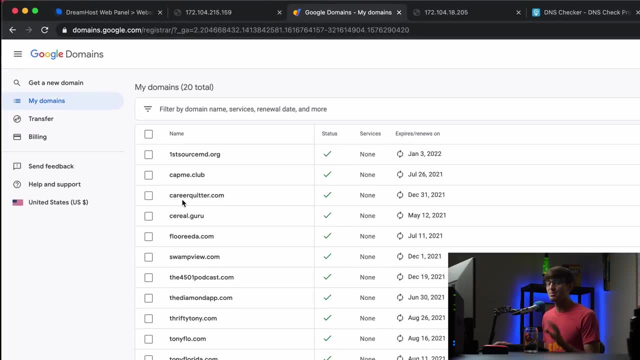 Different, different, different Hosting or different domain name registrar, but same process. Okay, so we want to find the domain name that we want to forward or not forward to, to map to an IP address. So careerquittercom, that's the one we want to work with here. 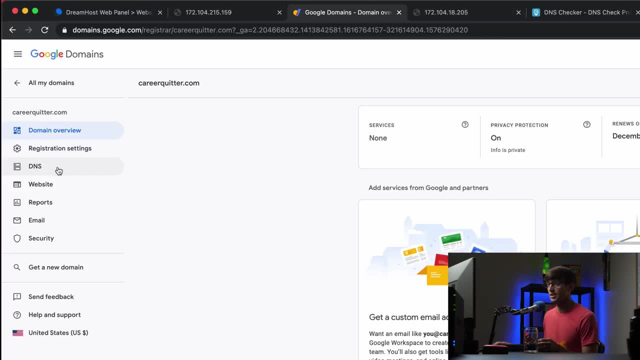 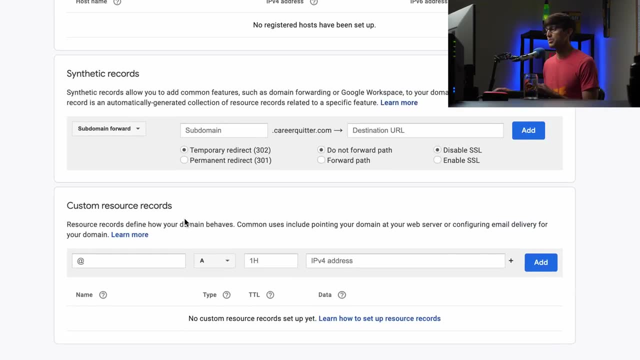 So let's click on that, Find the DNS settings Here. they are right here on the left, and we want to go down to the custom resource records section. in this case. So same thing as before. we want to take the bare domain name, which is careerquittercom. 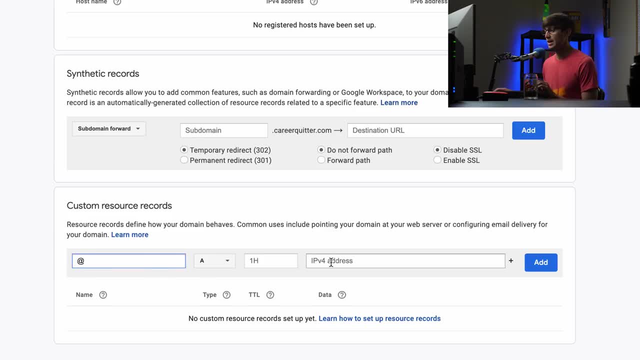 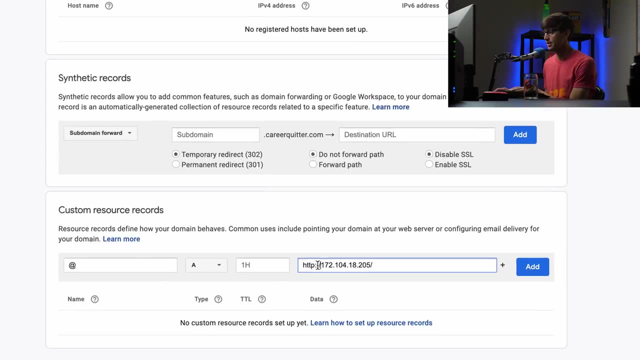 We'll use the at symbol for the shorthand and point it to an IP address, And that IP address is this one right here, the one ending in 205.. So let's put that in here. get rid of the everything else except for the IP address. 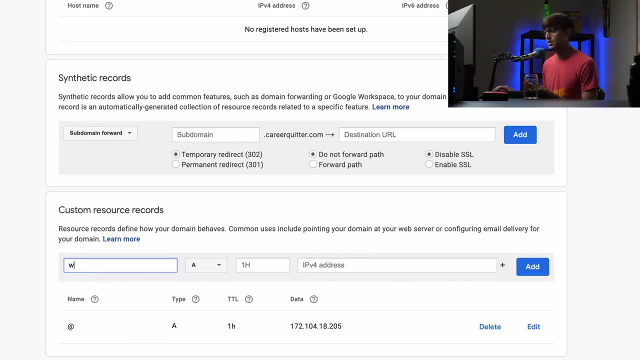 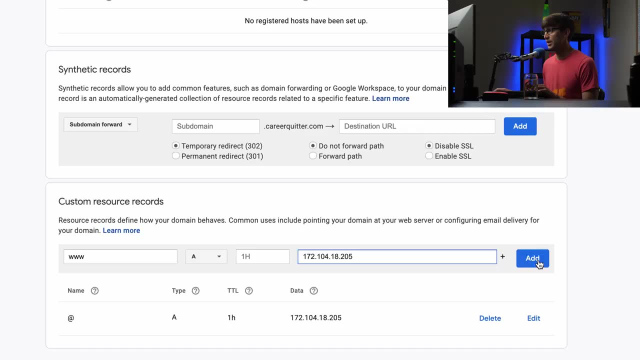 So we'll add that. And then we want to do the same thing for wwwcareerquittercom and point it to the same exact IP address. So we'll add that. And you know, you see this message up here changes. 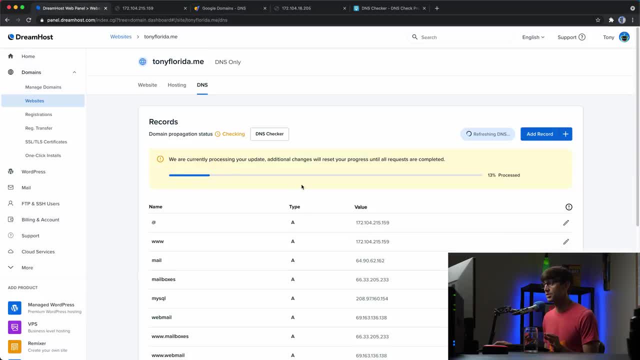 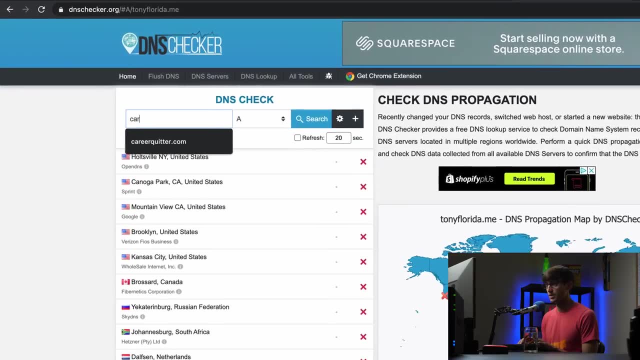 Okay, So let's let's check on the status here. So dream host is still processing the changes. I did not expect that to take that long, but we'll bear with it. Let's do the DNS checker for careerquittercom. 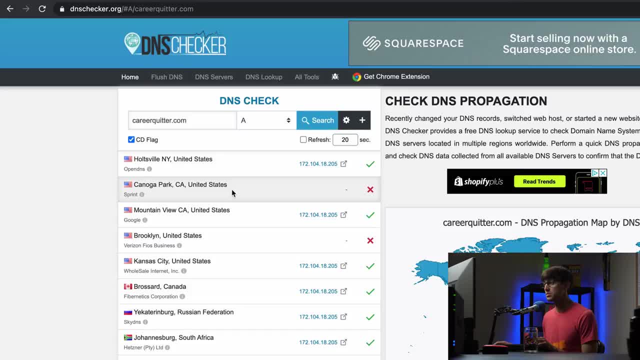 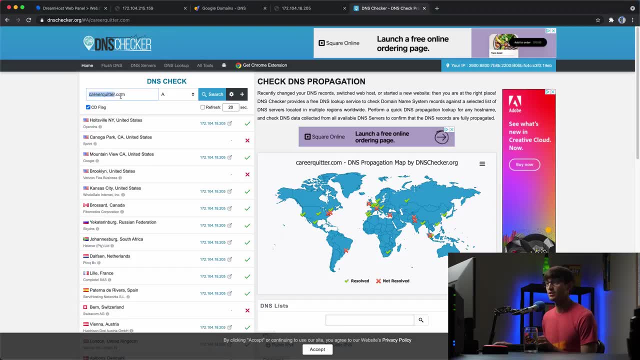 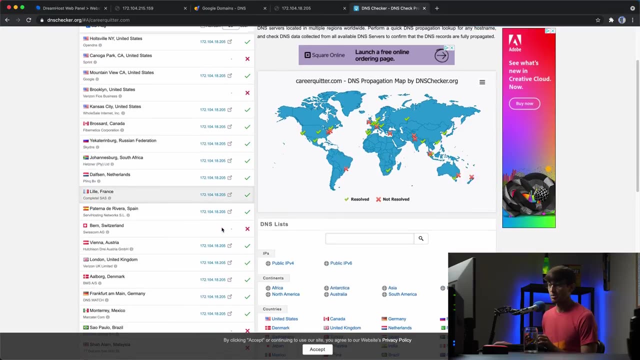 See if the a record has been updated and it's looking pretty good. So most of the DNS servers around the world have seen that update. So now careerquittercom is pointing that to that IP address for most of the DNS servers And I think it's probably fair enough at this point to test it out. 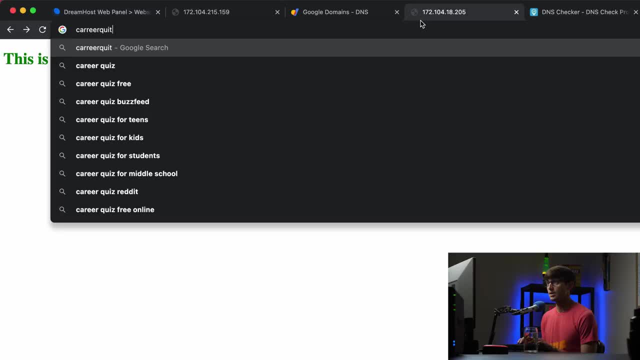 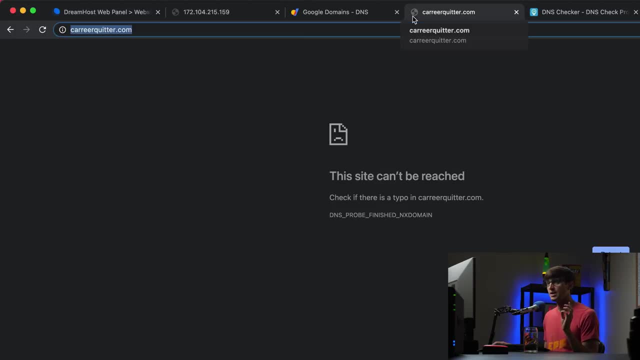 So let's go to careerquittercom, and that does not work. Um, but I might run into this too, because there's um and I actually spelled it wrong: C-A-R-E-E-R. quitter. Okay, there we go. 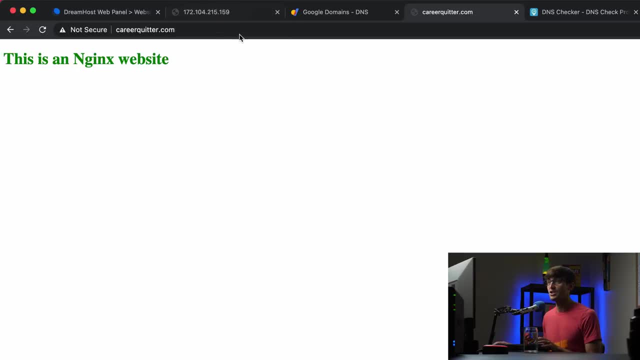 I was just going to say if. if you see something like that happen, it could be a caching issue. So what I recommend in those cases are to open up a guest window or an incognito window to to avoid all of those caching issues. 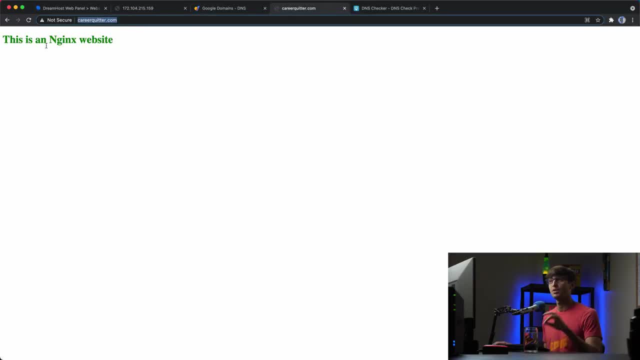 So, um, we're good to go, though. So careerquittercom now points to the same exact website that we saw at the IP address before. Um, and There's really nothing. well, there's one other thing, which is like a slightly advanced technical topic, that you might want to do if you are working at the web server level. 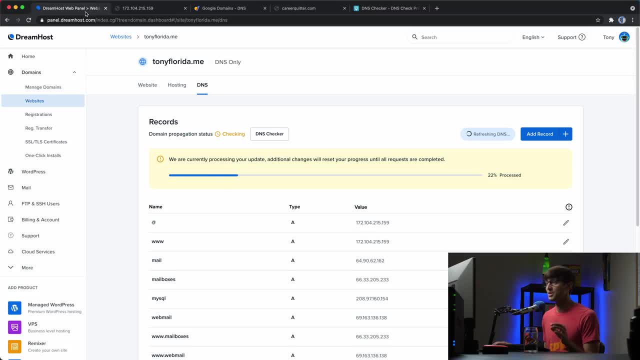 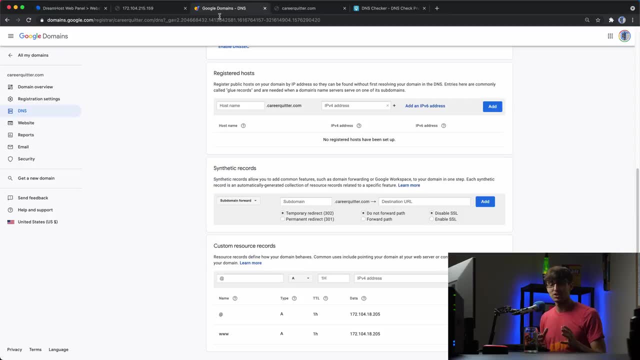 But if not, you're pretty much good to go at this point. uh, DreamHost is still processing the update. Uh, so let me, let me move forward and show you, um, if you are working with Apache and nginx at that level, uh, how to complete this, this, um, this update for your domain name. 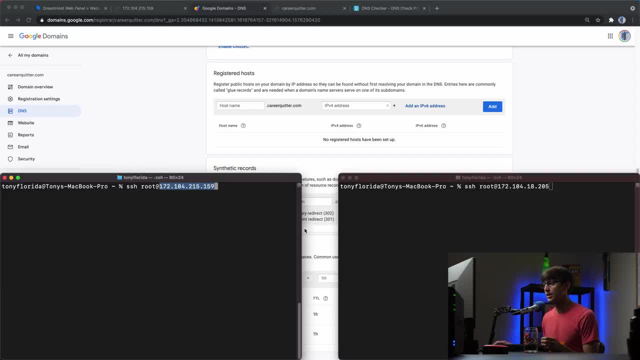 So, uh, what I do have is I'm going to go to uh terminal sessions here, um, and I'm going to log into those servers. Let me, let me make it the point clear here Again. if you are just here to you know, learn about DNS, a records. this is probably more than you need to know. 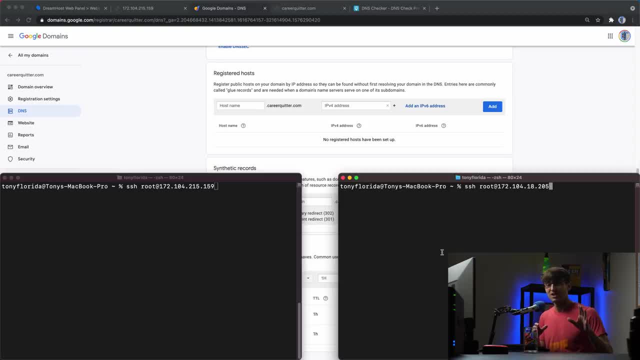 So you're probably good to go at this point, But if you do want to learn about Apache and nginx and how to configure, uh, your, your server with the domain name, then, um, please continue watching. So let's log into the server. that has. 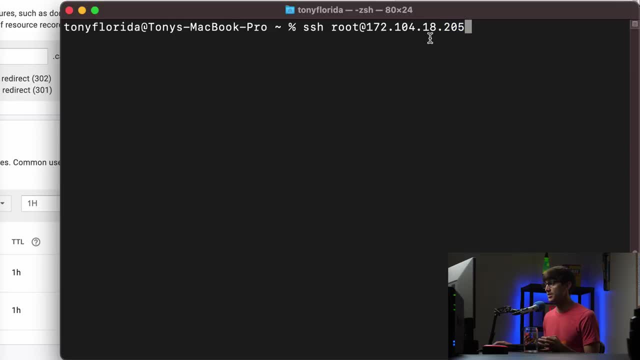 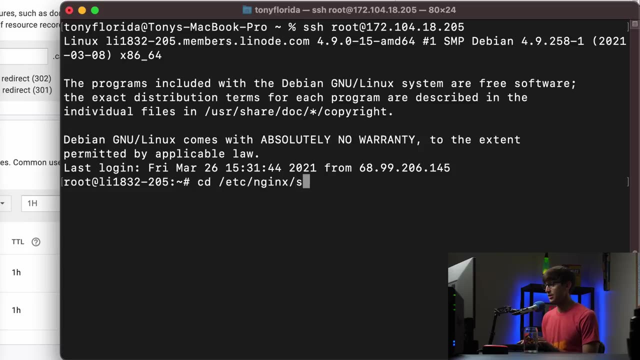 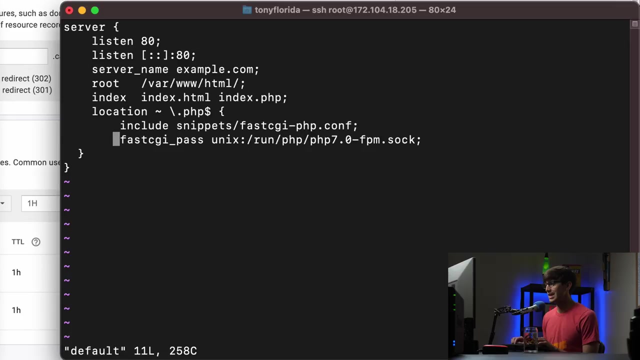 Um two Oh five, dot two Oh five. That's the nginx server here, And what we're going to do is go into the ETC nginx sites available directory, which is where my configuration file is for this website, And really all we're going to do in here is edit that configuration file and change the server name um from whatever it is right now to career quittercom. 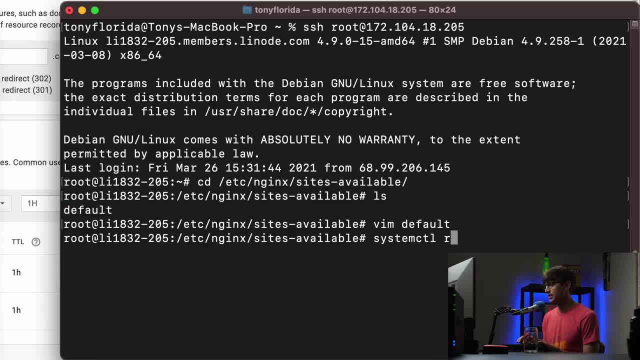 We'll save that And Do a system CTL, restart nginx. And now, from the perspective of the web server, um, it knows what type of requests when. when it sees requests from career recruitercom coming into the web server, it knows explicitly how to handle that request. 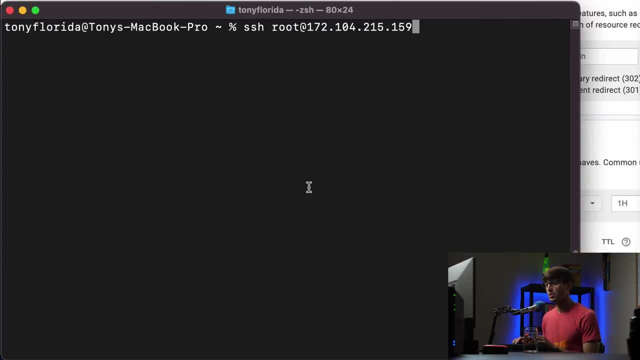 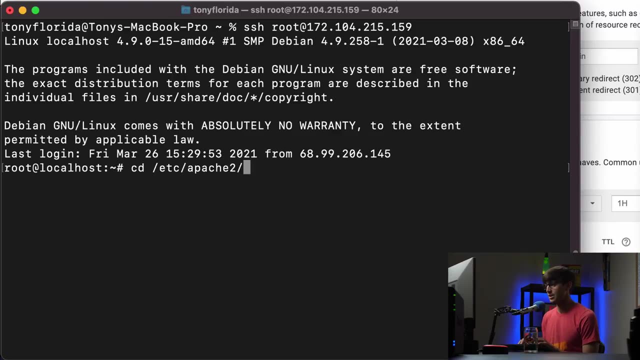 And we'll do the same thing for Apache, even though we're still waiting for that to update. We'll log into the Apache server ending in dot one, five, nine, Uh, we'll go into the ETC Apache directory, Apache two directory and then same type of structure sites available in here. 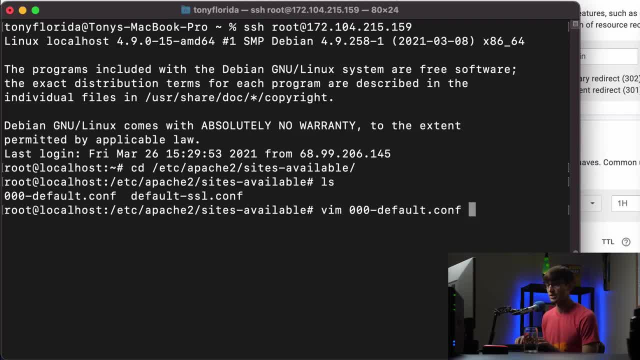 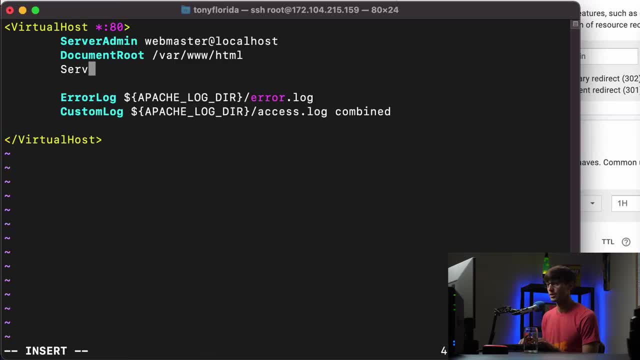 We want to edit the your, your configuration file. For me it's the default zero, zero, zero, dash, default configuration file And here, um, this is going to be server name and then it's going to be um. we're working with Tony Florida, dot me. 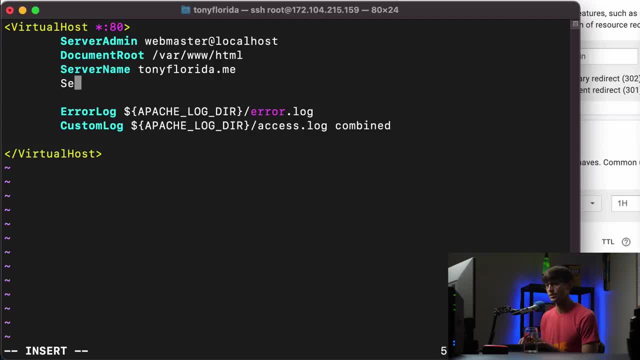 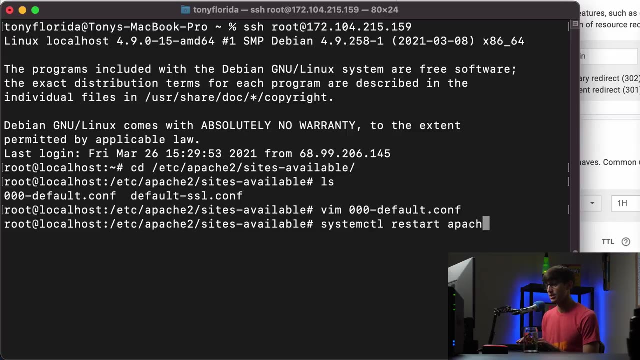 And then you can also do a- and I should have showed you this- on nginx server alias. It's going to be wwwtonyfloridame, So we'll save that. We'll do a system CTL, restart Apache two. Okay, And just to be explicit, let's go back into this one on nginx side. 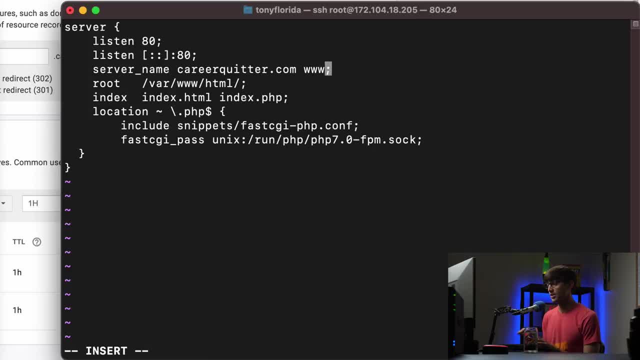 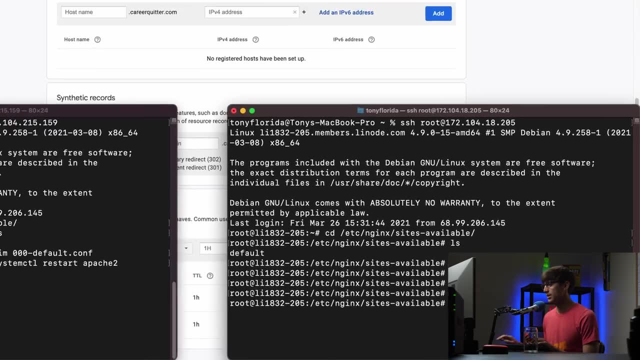 Uh, if you want it to add the www version here, you do www on the same line, dot career quittercom. Save that, We'll restart that again. Um, let's check on the status here. It's still processing the update. 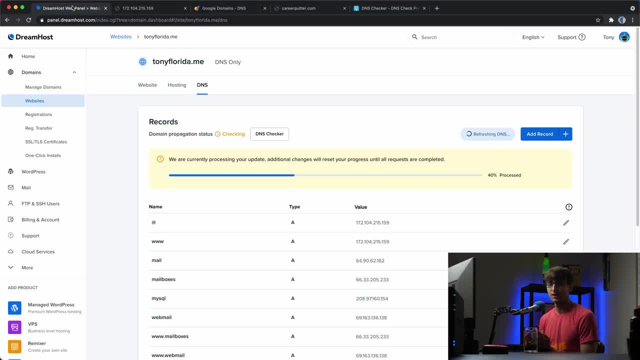 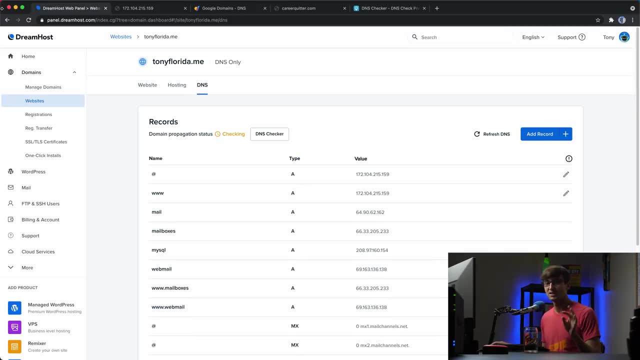 So let me pause the video here. Uh, when this finishes, we can verify that tonyfloridame is pointing to the correct IP address. Okay, guys, I'm back about 15 minutes later and the DNS has been set up on dream host for tonyfloridame. 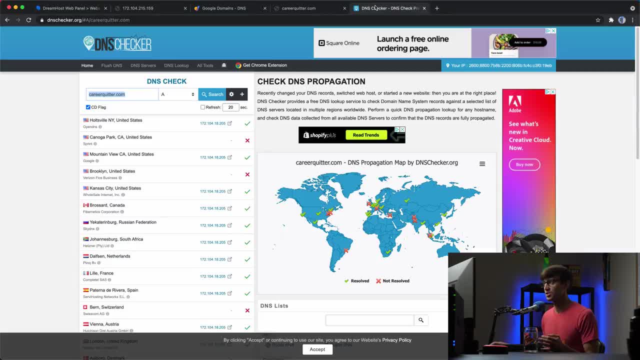 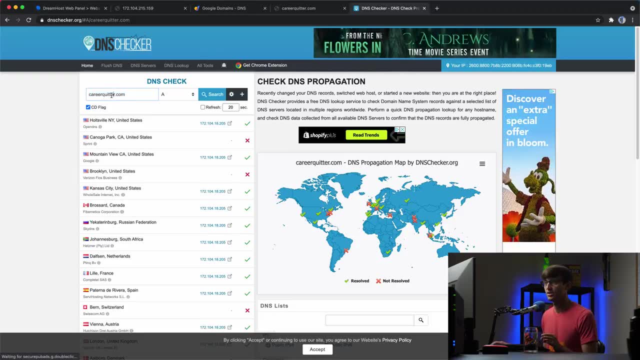 As you can see here. uh, let's go ahead and check that out with the DNS checker first. And uh, uh, while we're in here, let's, um, let's see how the DNS propagation has uh, progressed since last time.